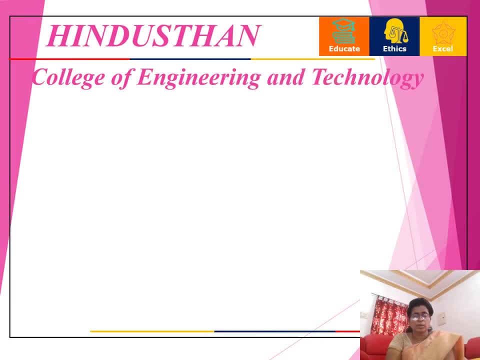 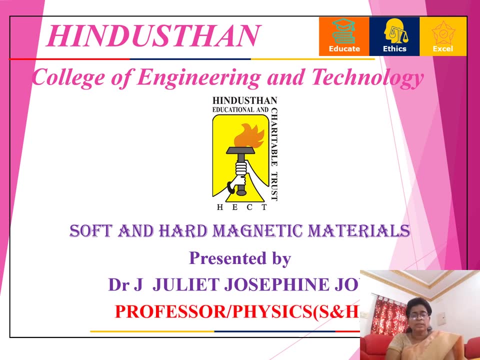 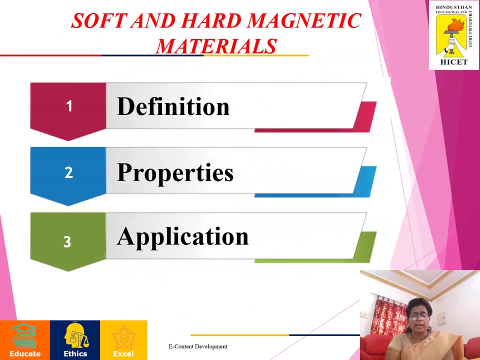 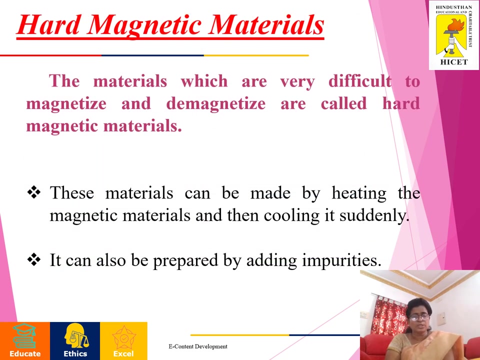 Welcome friends. I am Dr J Juliet Josephine Joy, Professor of Physics from Hindustan College of Engineering and Technology. In this video I am going to explain soft and hard magnetic materials and their definition, properties and applications. First we have to see what is hard magnetic materials. 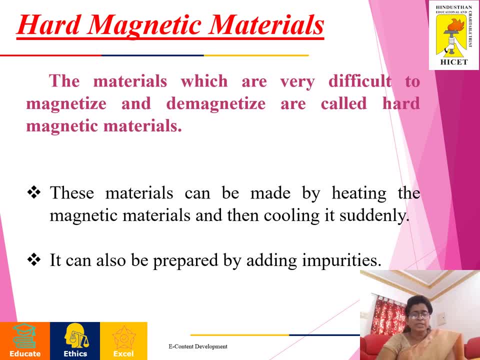 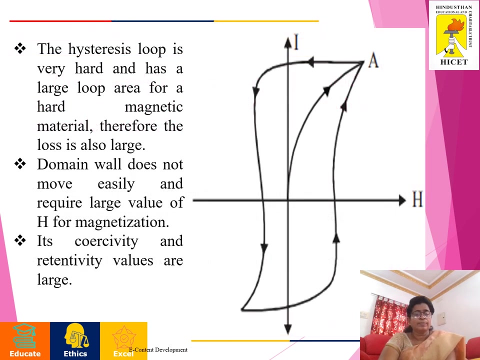 The materials which are very difficult to magnetize and demagnetize are called hard magnetic materials. These materials can be made by heating the magnetic materials and then cooling it suddenly. It can also be prepared by adding impurities. The hysteresis loop is very hard and has a large hole. 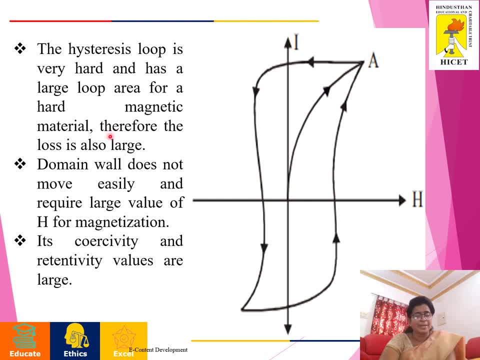 It is also a large loop area for a hard magnetic material. Therefore loss is also large. Domain wall does not move easily and requires large value of hutch for magnetization. Its cohesivity and retentivity values are large. Its eddy current loss is also high. 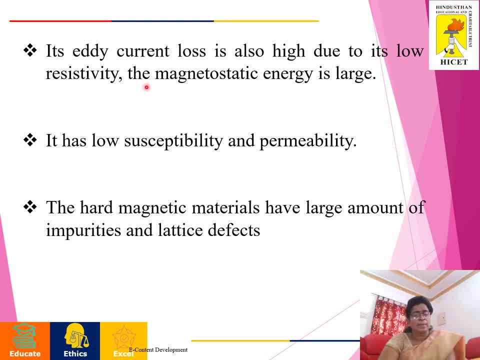 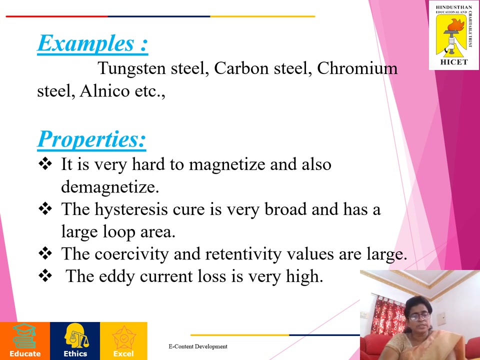 Due to its low resistivity. the magnetostatic energy is large. It has low susceptibility and permeability. The hard magnetic materials have large amount of impurities and lattice defects. Examples: tungsten steel, carbon steel, chromium steel, etc. 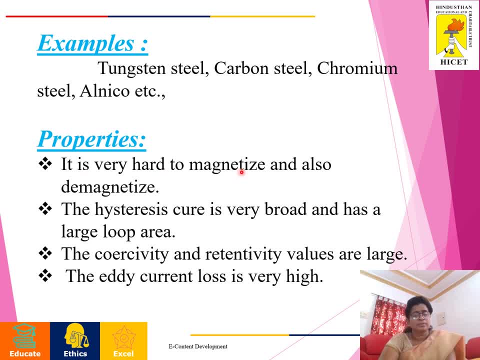 Properties. it is very hard to magnetize Properties. it is very hard to magnetize And also demagnetize. The hysteresis curve is very broad and has a large loop area. The cohesivity and retentivity values are large. 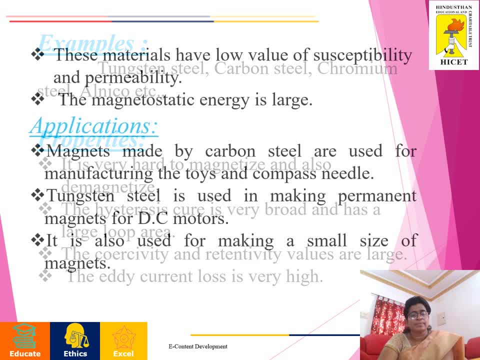 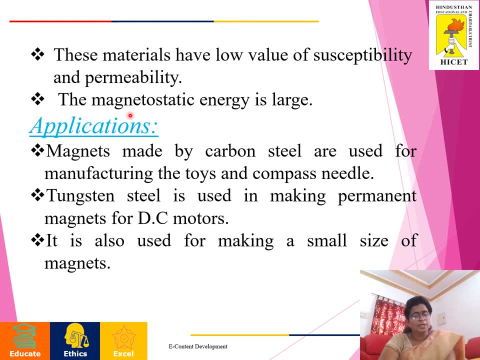 The eddy current loss is very high. These materials have low value of susceptibility and permeability. The magnetostatic energy is large Applications Magnets. Magnets made by carbon steel are used for manufacturing the toys and compass needle. Tungsten steel is used in making permanent magnets for DC motors. 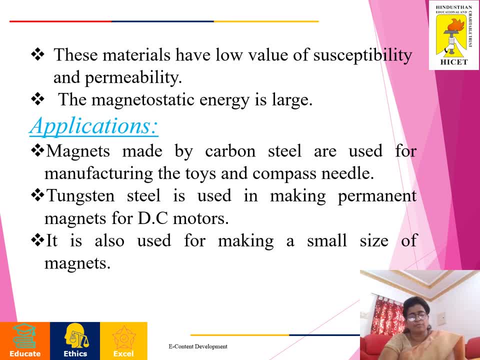 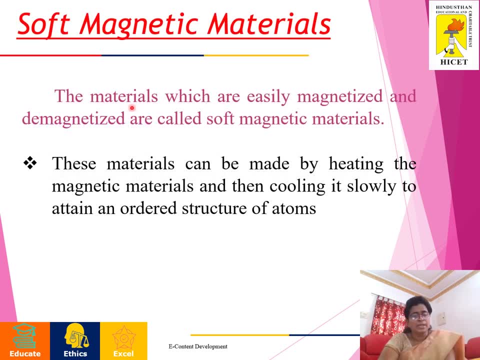 It is also used for making a small size of magnets. Then we have to see soft magnetic materials. The materials which are easily magnetized and demagnetized are called soft magnetic materials. These materials can be made by heating the magnetic materials and then cooling it slowly to attain an ordered structure of atoms. 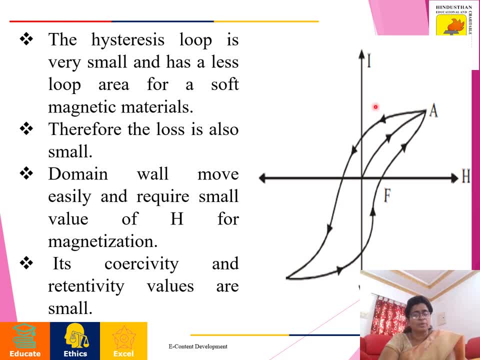 The hysteresis loop is very small and has a less loop area For hysteresis soft magnetic materials. therefore loss is also small. Domain wall moves easily and requires small value of hutch for magnetization. Its cohesivity and retentivity are small. 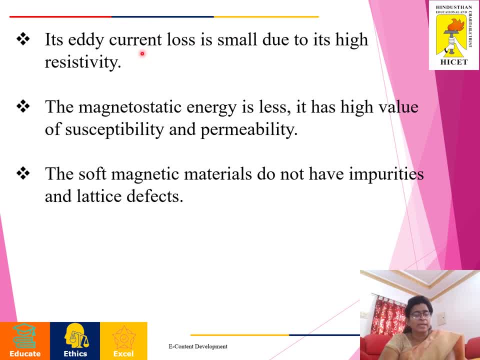 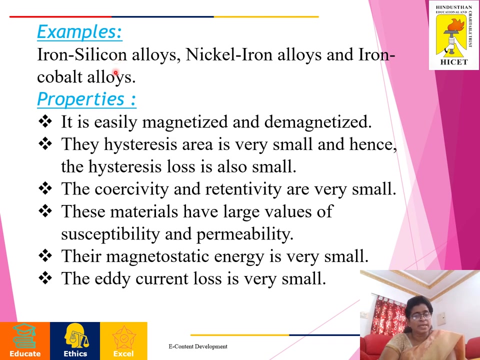 Its eddy. current loss is small due to its high resistivity. The magnetostatic energy is less. It has high value of susceptibility and permeability. The soft magnetic materials do not have impurities and lattice defects. Example: iron-silicon alloys, nickel-iron alloys, etc. 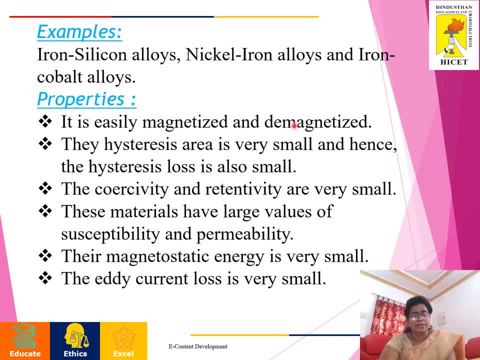 Properties: It is easily magnetized and demagnetized. The hysteresis area is very small, Hence the hysteresis loss is small. The cohesivity and retentivity are small. These materials have large values of susceptibility and permeability. 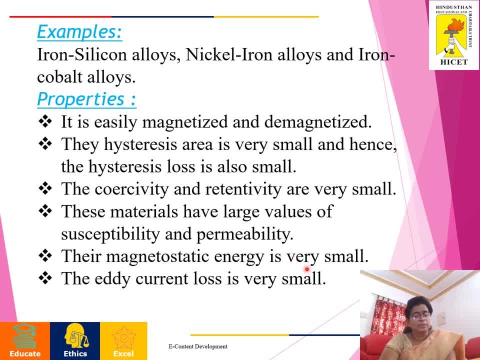 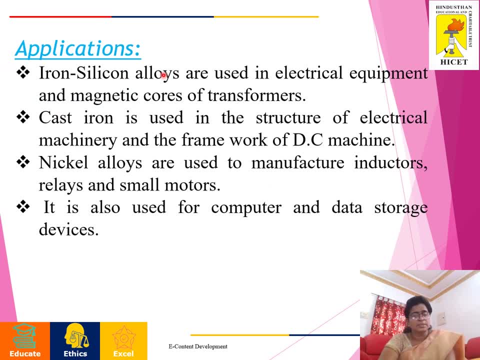 Their magnetostatic energy is very small. The eddy current loss is very small. Applications: Iron-silicon alloys are used in electrical equipment and magnetic cores of transistors. Cast-Ion is used in the structure of electrical machinery and the frame work of DC machine. 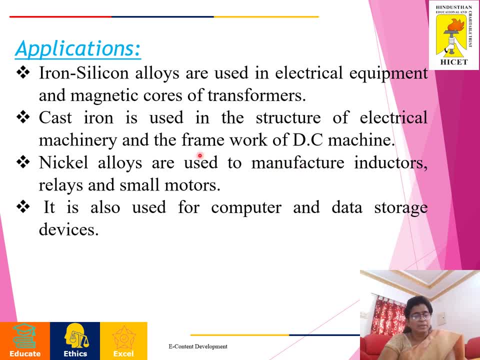 Nickel alloys are used to manufacture inductors, relays and small motors. It is also used for computer data storage devices. Thanks for watching. Thank you.